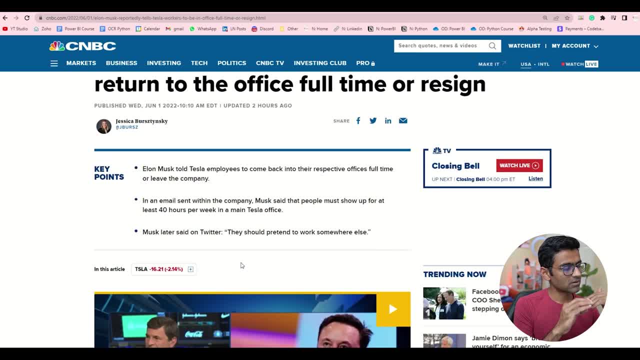 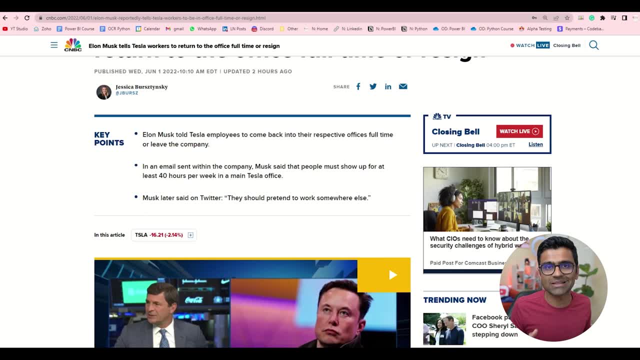 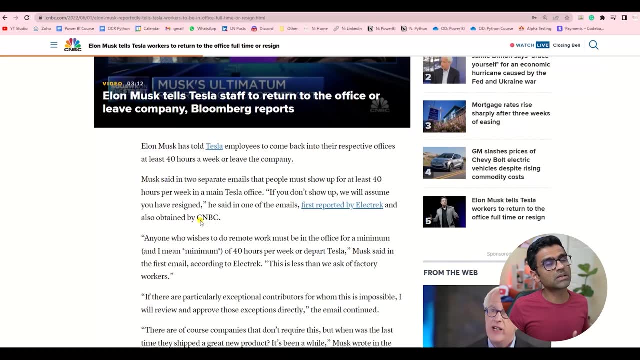 and when I go to any news, you will see this tag. you know that for the news. it knows that this is the news of company Tesla. Now CNBC editor might be putting this tag explicitly, but I think the better example is something like Google News, where they are an aggregator website. 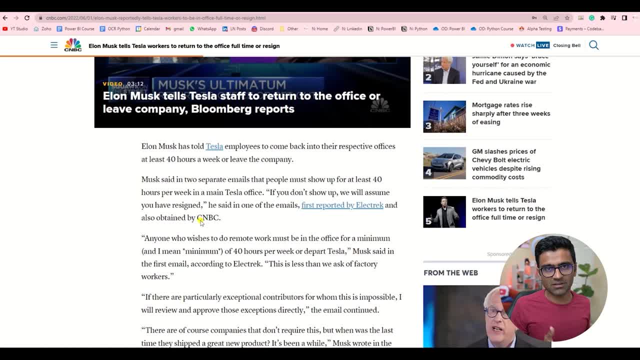 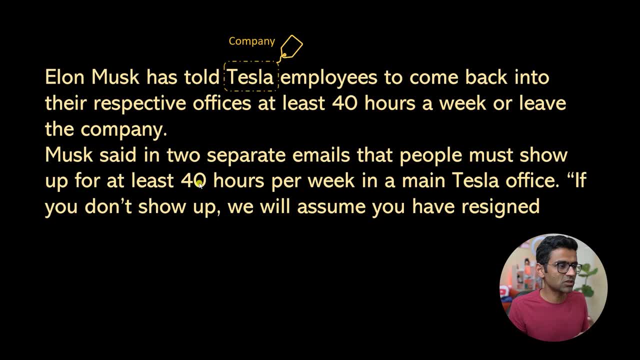 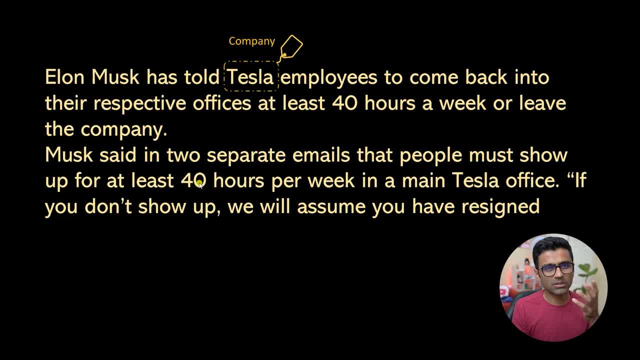 Let's say I want to search for a company. Let's say I want to search for a company. Let's say I want to search for a company: Tesla as a company. Now you might think: oh, this is easy, all you can do is just search for company. 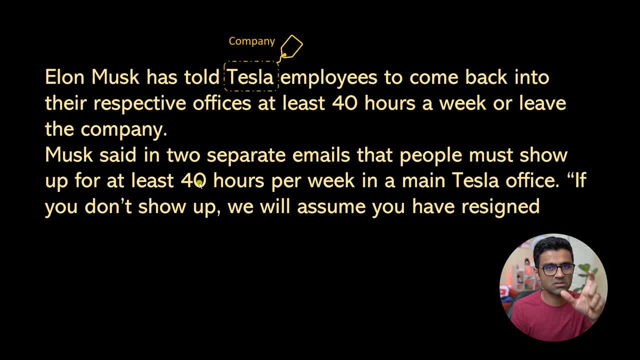 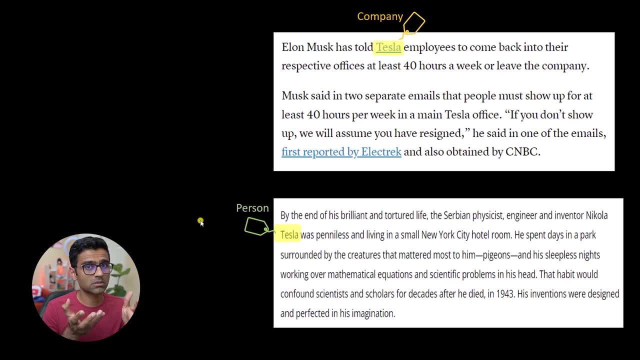 Tesla or any other company. You can have 20 000 different companies and just search for it, But it might not be that straightforward, because Tesla could be a name of a person also. You know Nikola Tesla, a genius scientist. So when I see a term Tesla in any blog or any article, I don't know if. 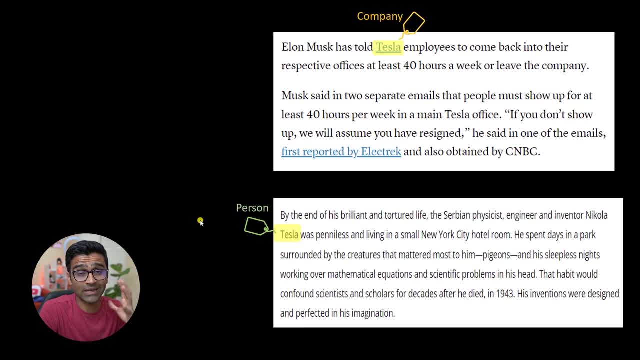 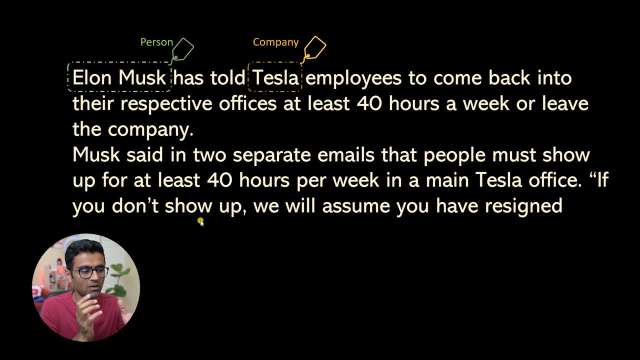 it's a person or company. So that's when the NER system can be useful, where the system actually tells you what entity it is. Okay, so NER is basically named entity recognition, where you try to extract different entities in your text. So here, Elon Musk is a person. 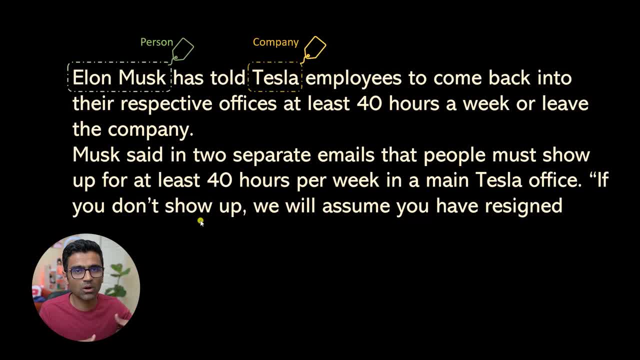 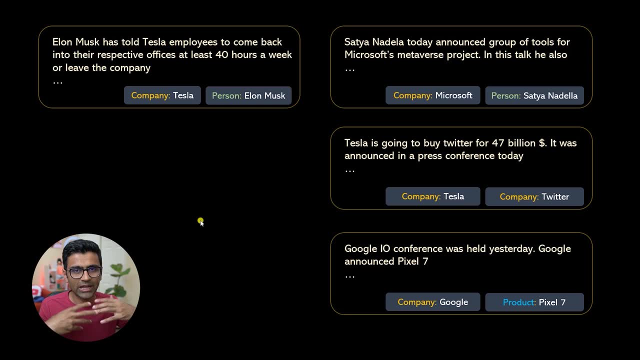 Tesla is a company. There could be a location like New York, India. These are locations, Money things, like company names. this could be anything. But when I see a lot of articles- Let's say, you're building a website such as Google News and you have a lot of articles and you don't- 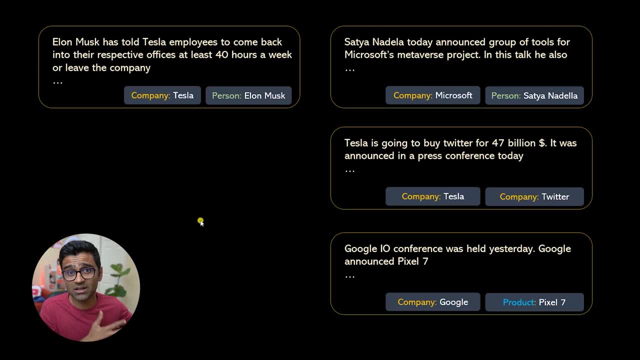 know which entities are mentioned. maybe you can use NER system and it will extract all the entities. See here I have shown different example where companies products. even look at this example where Beijing 7, is a product, So the entity product. here there are two entities, Tesla and Twitter. so if you can extract, 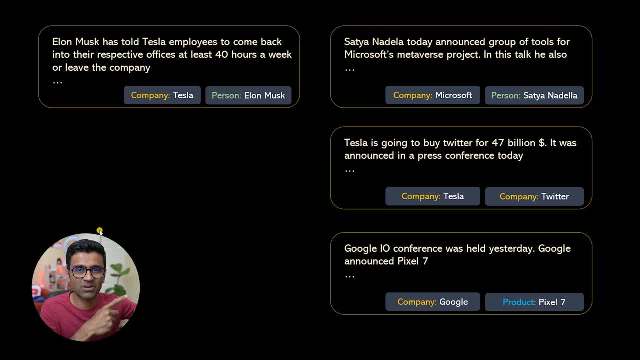 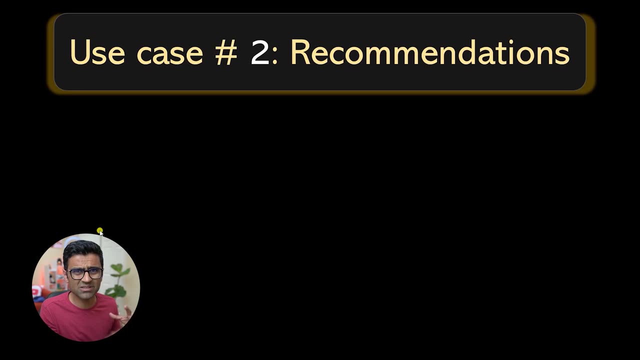 these entities. then you know, in the CNBC example we saw, if person can type in just name of the company or name of the product, we can show you all relevant articles. so this is very useful in case of search. the other use use cases: recommendation, which is associated with the first use case, we, which we already 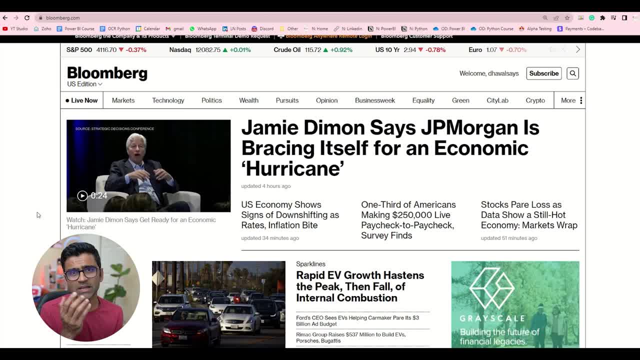 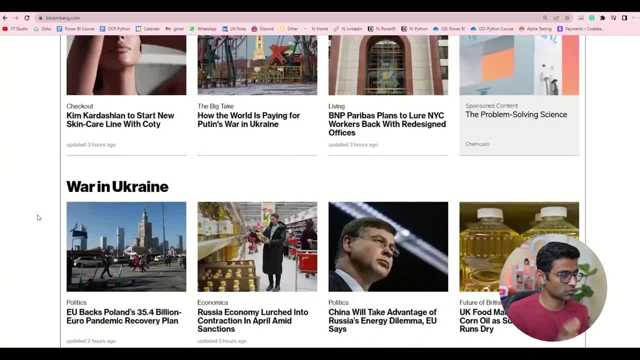 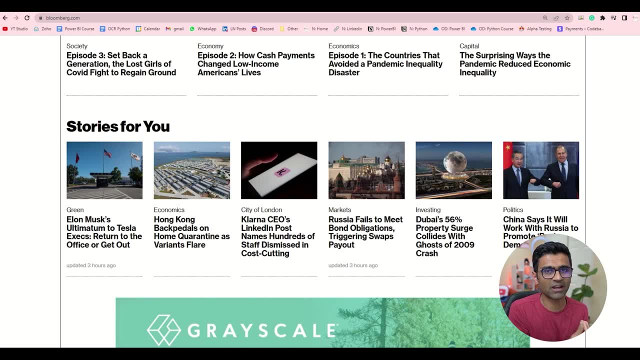 mentioned. you might have seen on many website, for example, on Bloomberg News, I see this section where it says stories for you, which means these are the stories which they are showing based on my preferences. this is a recommendation system. so here let's say, I have read article about Elon Musk or Hong Kong. 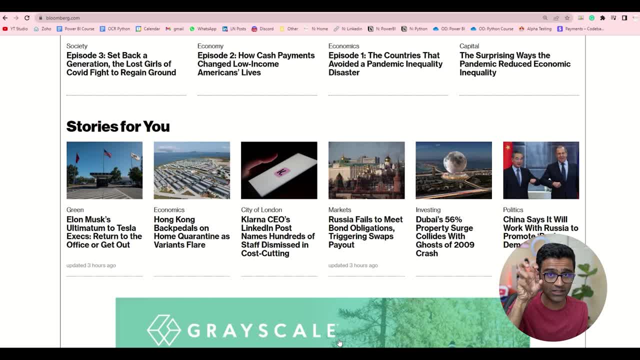 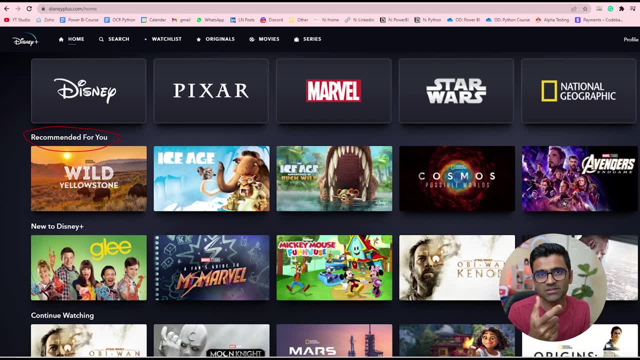 before then from that article. let's say, if the entities are Elon Musk, location is Hong Kong, and if I like to read such an article, it will show me similar articles or having a similar entity, same like news- not news, but the movie recommendation system. I have Disney subscription and I like to watch National Geographic documentaries. 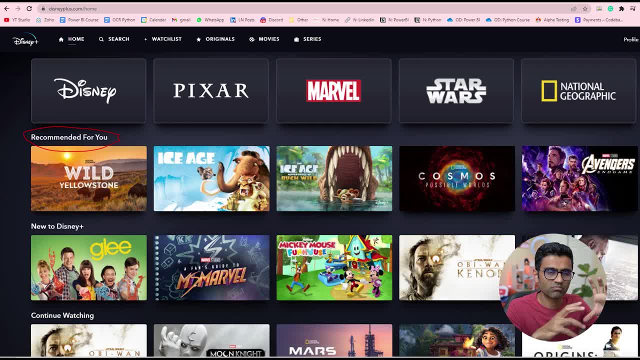 so here, when you are looking at a documentary, the entities could be: who is the production house? is it Mar-a-Lago, Pixar, National Geographic? who are the actors in the movie? right, so these are production house actors. these are various entities and if I have a preference of watching movies from certain actor or certain production, 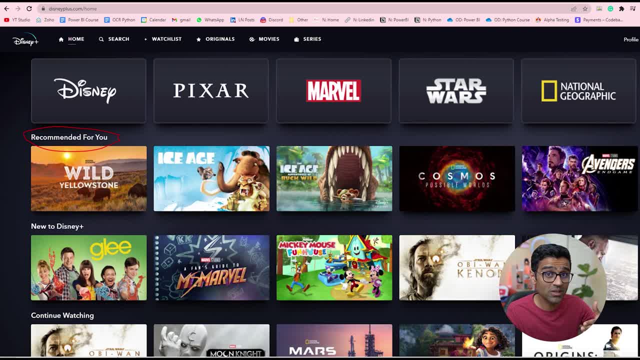 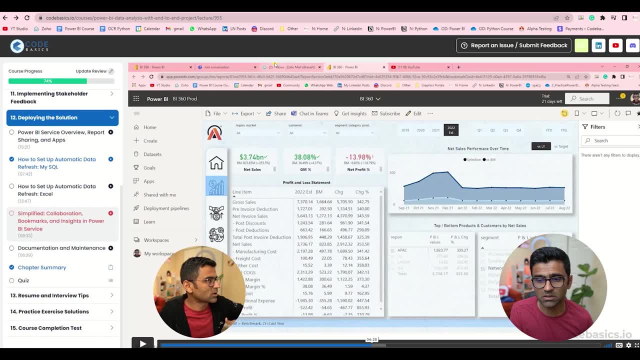 house. then the recommendation system can show me the movies or documentaries from those preferences. the third use case is customer care service. I build this website called coldbasicsio for it's it's a learning portal. basically, I have a program and here is an awesome course I have out on Power Bi data. 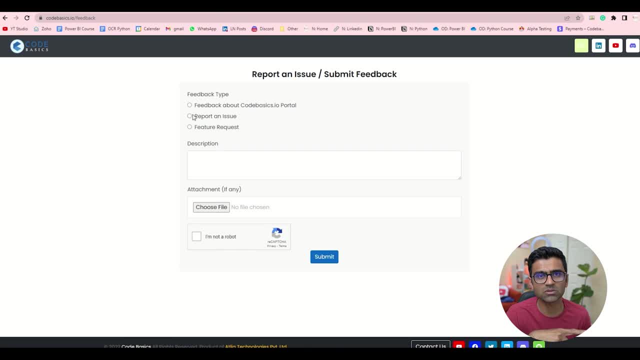 analytics and there is a report issue button. so if someone is facing issue in my course, they can report an issue. okay, now see, this can be made simple by right now. I know you are in Power BI, because I know actually that the issue is related to Power BI, but let's say, if I have a generic form where you can just 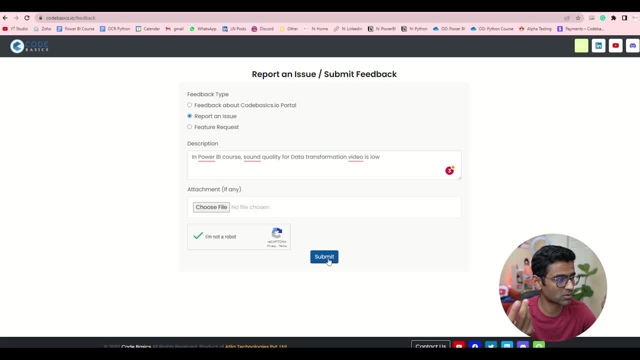 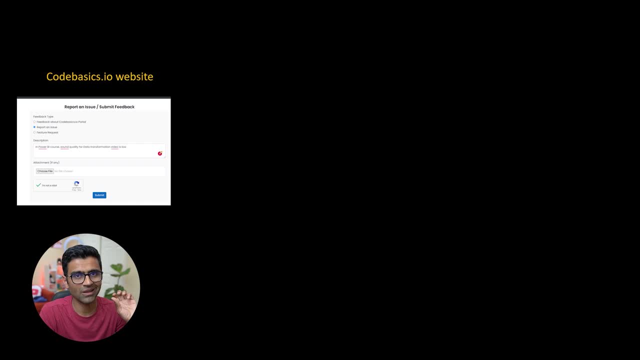 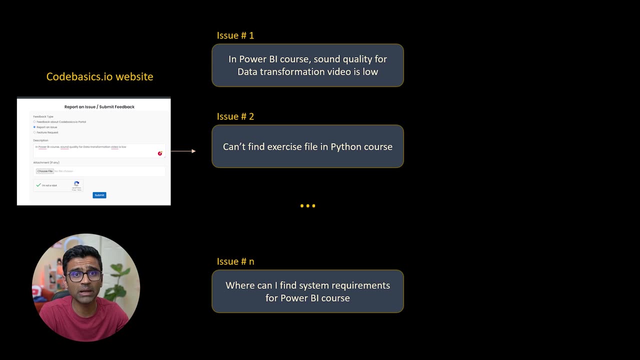 type in text and I don't know what course you're talking about. okay, then what happens like how do I know which course it is? so when you submit a query from code business code, IO website in the backend, I am getting these queries from many, many people. well, the reality is, we have not seen any major issues, so 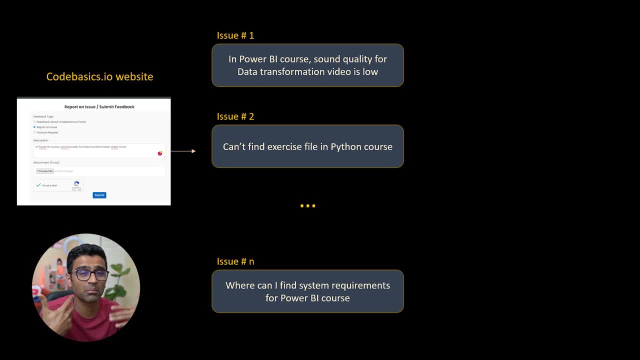 far. but let's say you are talking about big system where there are multiple people filing multiple complaints, and let's say you have separate customer support team. let's say, for Power BI course I have a separate team and for Python course there is another team and they both handle the queries related to 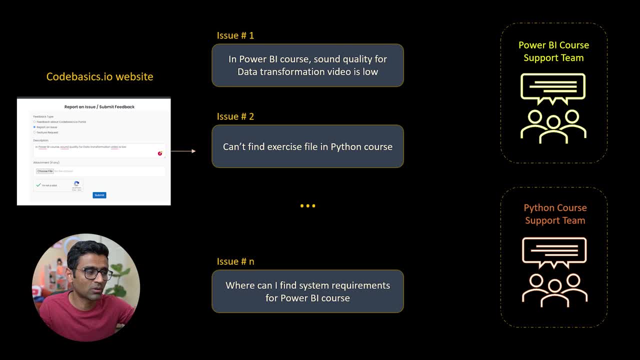 that course because they are trained to answer the queries in that particular course. now, if I can extract the entities which is a course- let's say here course is my entity- and if I can extract the course name, then I can route those issues to a relevant ticket. now you can have a drop-down, simple drop-down, in the. 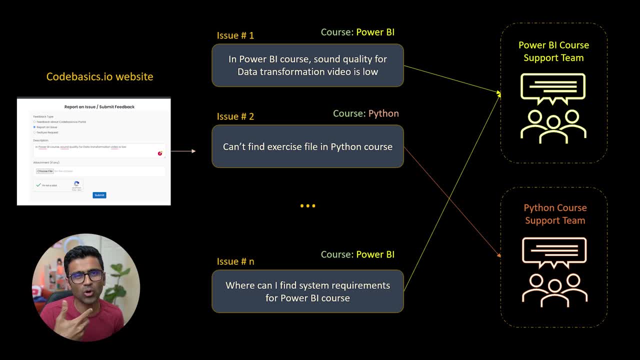 contact us form and you can have user selected. but if you auto detect that, then it's, it looks nice, you know. so it's, it's better, all right. so now let's open Jupyter notebook and write code in spaCy and we are going to use inbuilt NER system and then 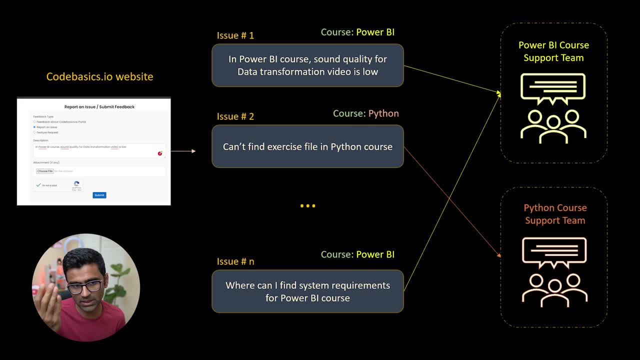 towards the end. we'll talk about how you can build your own NER system. we will now explore NER support in spaCy. as usual, I have downloaded NER support in spaCy. and I have downloaded NER support in spaCy. as usual, I have downloaded NER support in spaCy. as usual, I have downloaded. 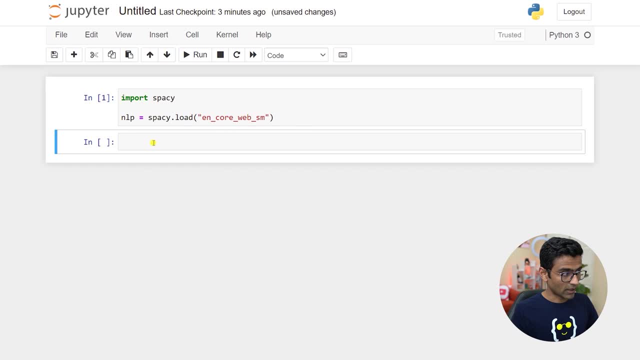 spaCy's English model, and now I am going to look at all the pipe names. so this shows you the the components in that NLP pipe, and we see a component called NER, so we'll see how this particular component works. you can have a statement like this: Tesla is going to acquire Twitter. it's kind of dangling. 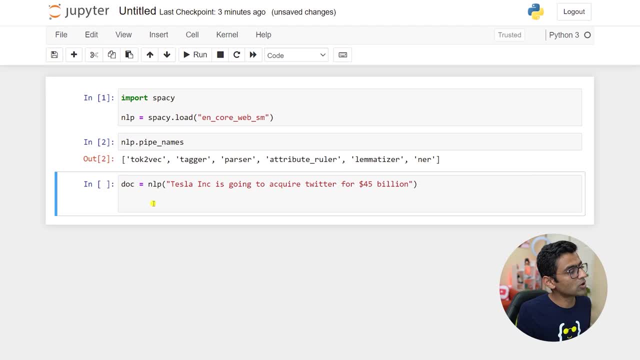 right now I don't know what's gonna happen. and if you want to look at all the entities here, you can say for entity in Docentities, so doctor entities contains all the entities in this particular statement, and then you can print the entity dot text. so that is the label and 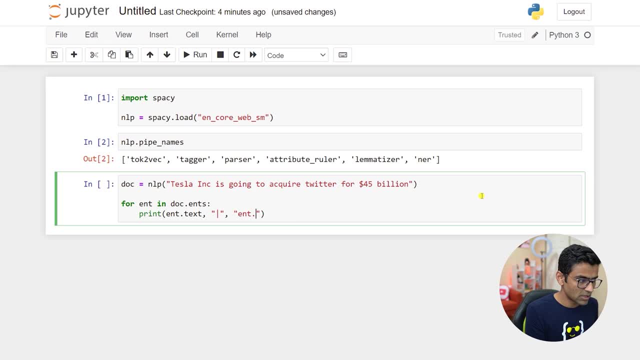 this was he and I was only starting out when the two images were in the production- this pipe operator. and then you can print ENT dot label. so this prints the actual label, whether it's a company, whatever, and also I'm going to. okay, let me just try this first. so it says: Tesla incorporation is 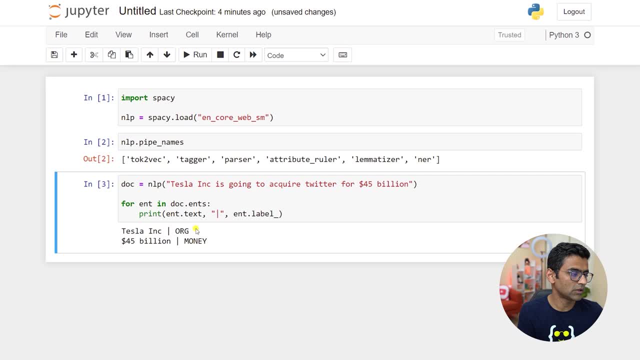 organization. 45 billion is money and if you want to see expanded version of this token, you can use spaCy dot explain. spaCy dot explain and then give label as an argument. it says arg means companies, money means monetary value, etc. you can use this placey. we have used this before in our tutorial, this placey to you know. 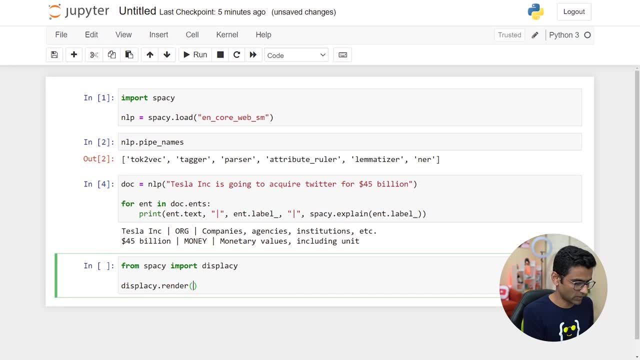 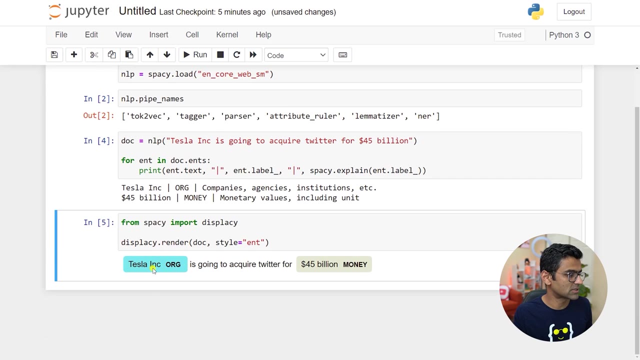 visually render the same thing in a better way. so it's the same thing. but I am saying style is equal to ENT, so display C dot, render the document, and the style I want is ENT. ENT means entities. so when I do that, see it says Tesla ENC is arg and Twitter 45 billion is. 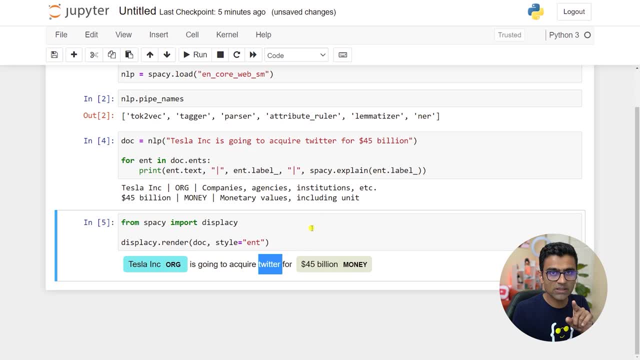 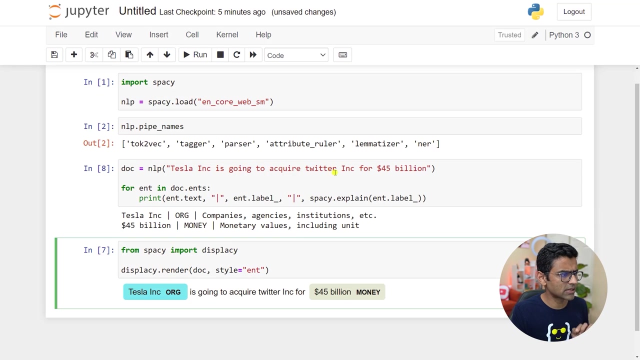 money. Twitter. it did not recognize because looks like spaCy is using some kind of rules or patterns to recognize companies. so if I say Twitter dot INC, that's a popular way of representing companies in US incorporation- okay, that did not work quite well. so now you're realizing here that, okay, let me try this. see Twitter. 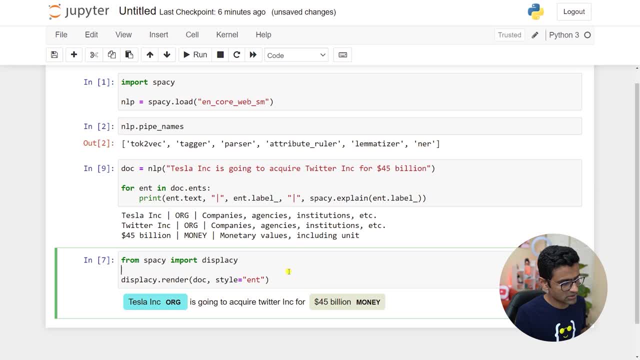 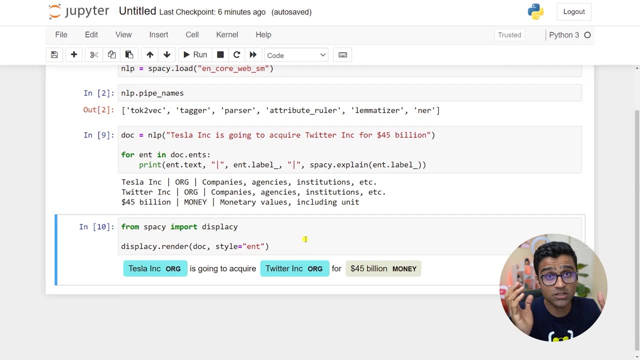 when I capitalized it it worked. so you are realizing that the spaCy is out-of-the-box named entity recognition is not perfect, and that's perfectly fine. it is using some kind of rules that if there is a word with first letter as capital, followed by INC, then that's a company. all right, we'll look into how you can. 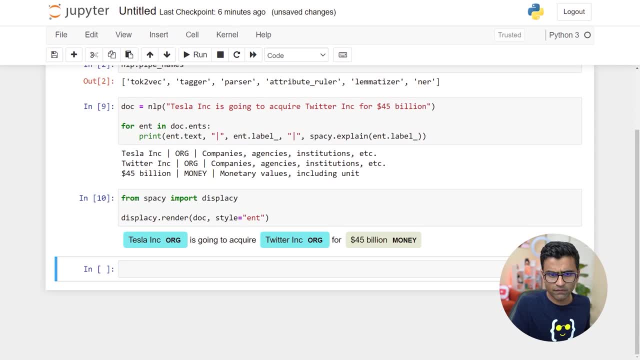 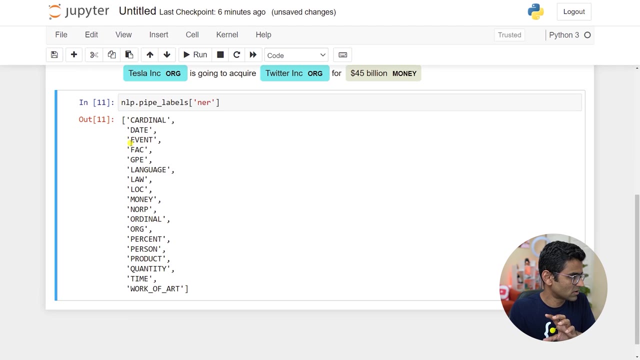 build your own model little later. but let's first see what all entities that specie supports. we just looked at org and money. if you try this particular instruction, it will print all the entities that specie supports with that particular model, with this particular trained model. okay, this model is a. 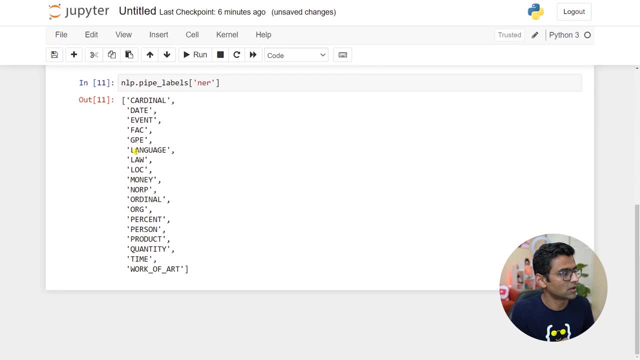 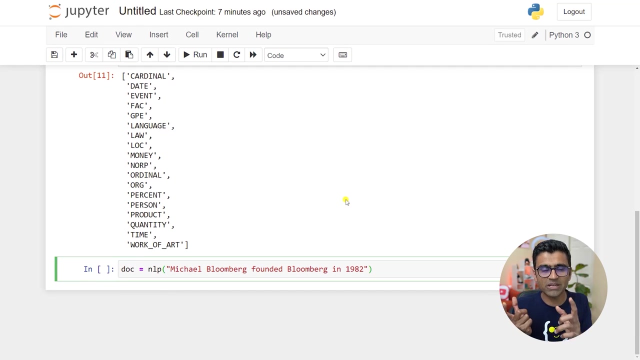 pre-trained model and that suppose these many entities. so language, money, percentage, product, even work of art and so on. let me try different step statement. I used to work for Bloomberg and Bloomberg was a company name, but Michael Bloomberg was a person who founded that company. so now 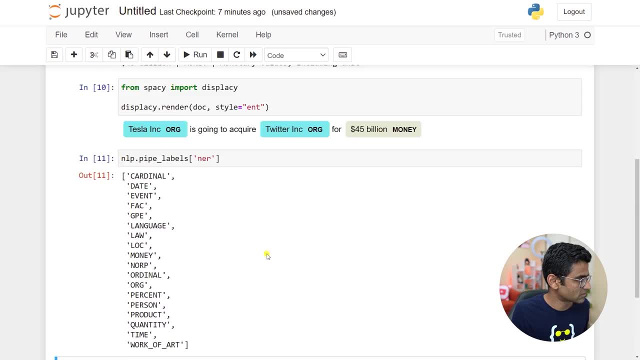 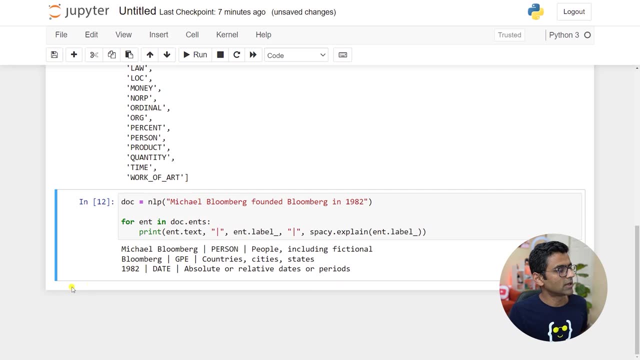 if you print the entities. so I will just use my most powerful weapon here, which is control C, control V, and it says: Michael Bloomberg is a person. this is now. this is wrong. okay, Michael Bloomberg, this it should have recognized as a company, but Bloomberg is saying GPE, if I do, Bloomberg, INC, maybe. 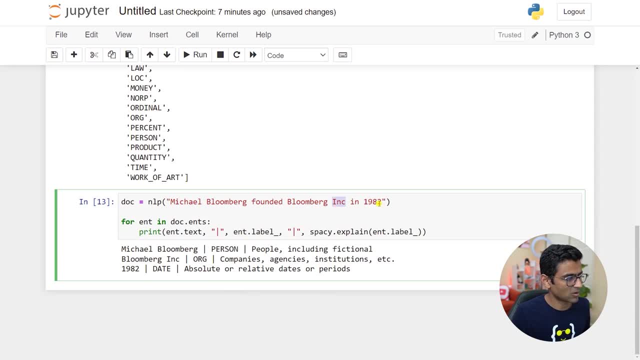 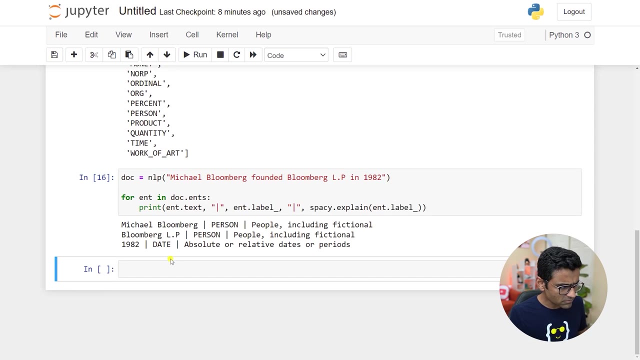 it will work. see now it says corporate company RL, dot P. okay, yes, this is funny. it's saying my Bloomberg LP is a person. so you are saying this is not perfect, but it works on many cases. in 1982 it said it is a date, so I want to try a different model now. so here in in Google you can say: 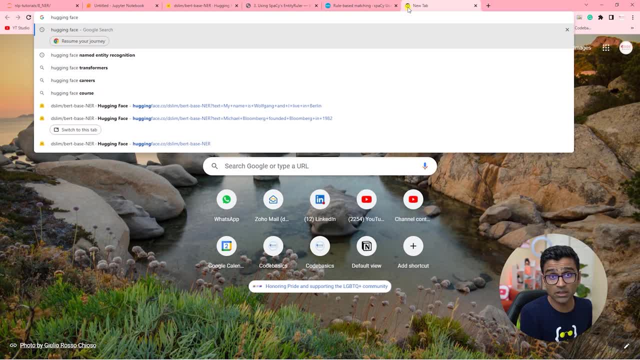 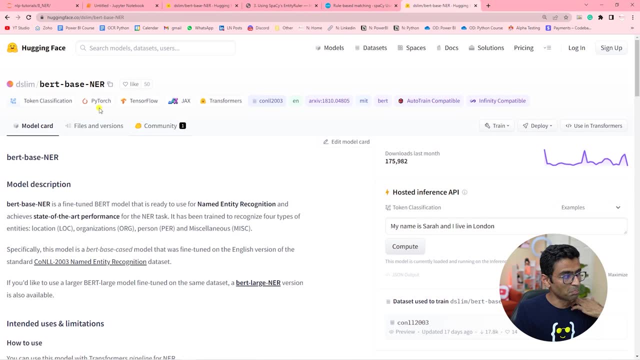 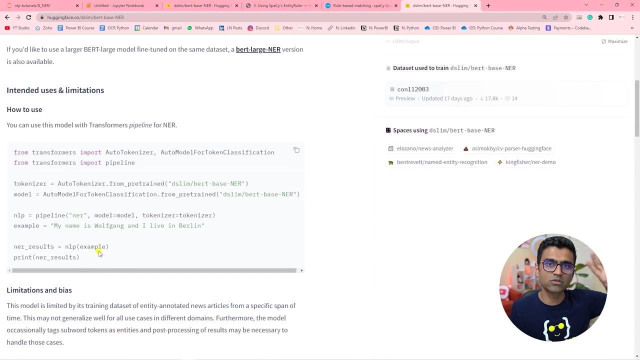 huggingface is a popular machine learning NLP library and you can say huggingface name entity recognition and they have some word based name entity recognition which you can try here. so here see, it is using this code which is huggingface. we use specie, but this particular model is used for three type of entities. 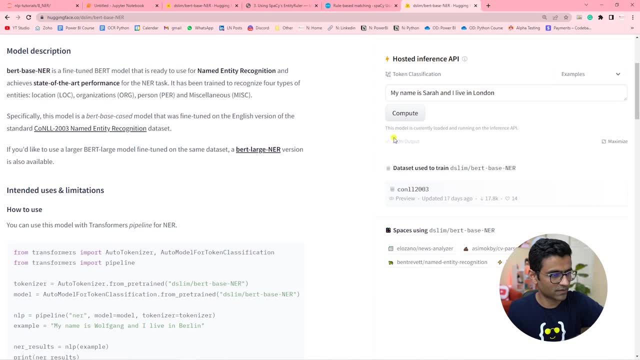 location, organization, person and miscellaneous four entities. and if you do compute, it says Sarah is a person, London is this. you can look at different example like right, like say this: see, Clara lives in California, so Berkeley, California, both of them it identified as a location. you can type your own thing. 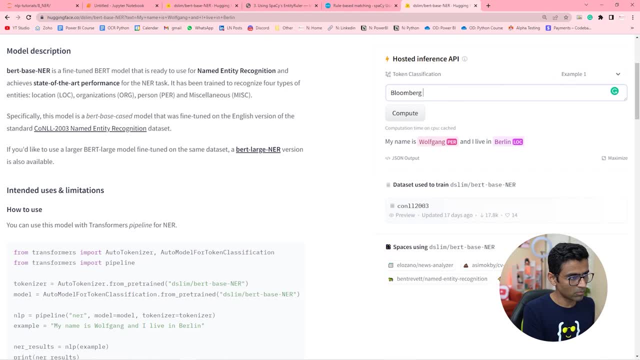 as well. you can say: Bloomberg founded Bloomberg in 1980. now, here again, see, this is making mistake. but if I do, because Bloomberg was Bloomberg, it is saying organization. the first one is actually person. see, now, Michael Bloomberg is person. so you're realizing that it depends on how we have trained the model. 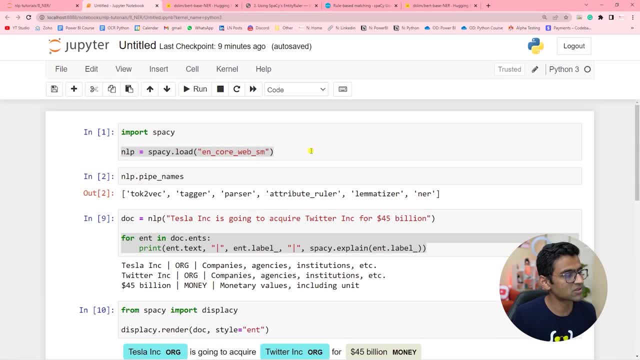 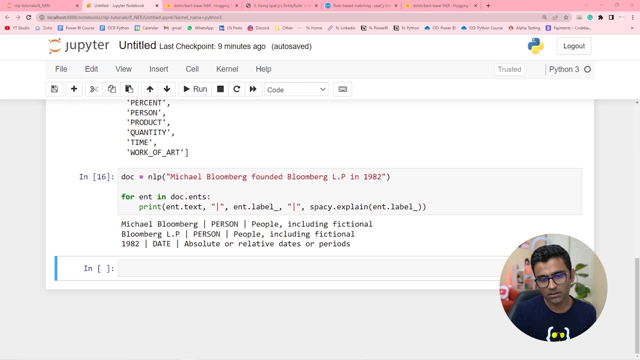 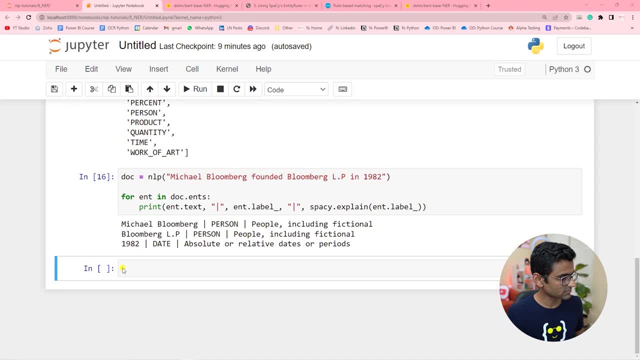 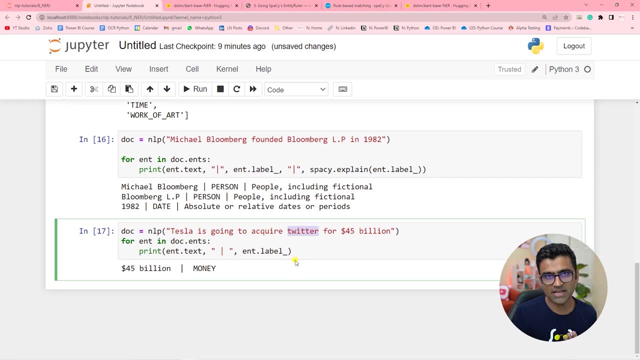 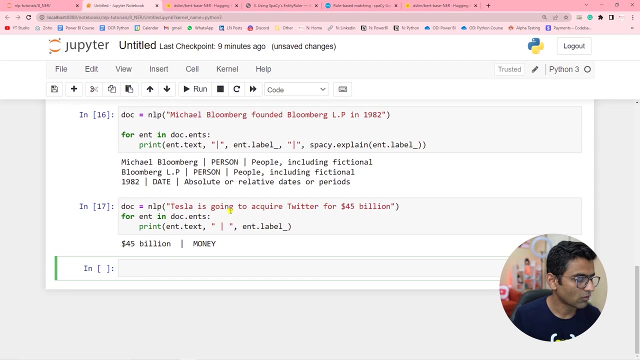 a custom entity. for example, here in this it is not recognizing Tesla or Twitter as companies. okay, and 45 billion is a money, so that's fine. now what if I want to add a custom entity to my model? and I want to add a custom entity to my model. 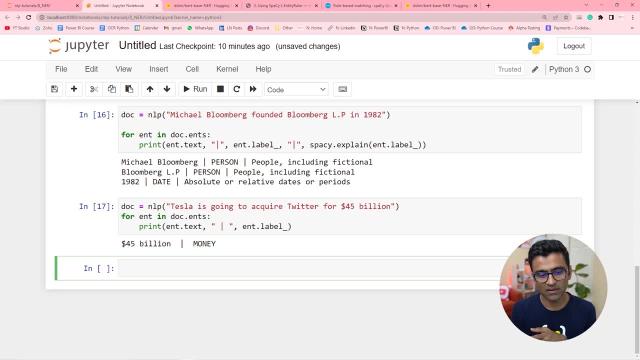 add those two entities specifically. I want to say that, hey, specie, these two are companies. okay, so you can do that. so let me first explain you a concept of a span. span not spam, so span is a class in specie. so when you are looking at for 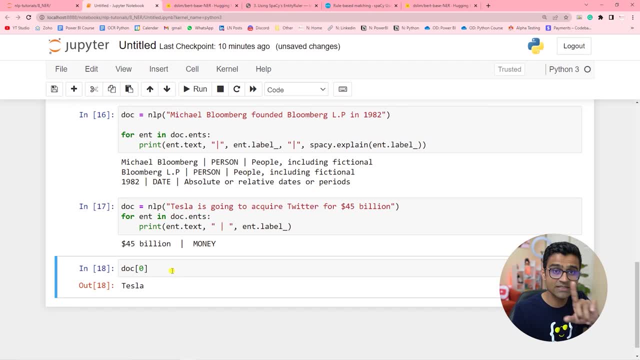 example, when you're looking at it, any single token. this is a single token and if you look at the type of this, it is a token, but using Python's slice index operator- let's say you said two to five- it is showing you a span of tokens like a substring going to acquire and 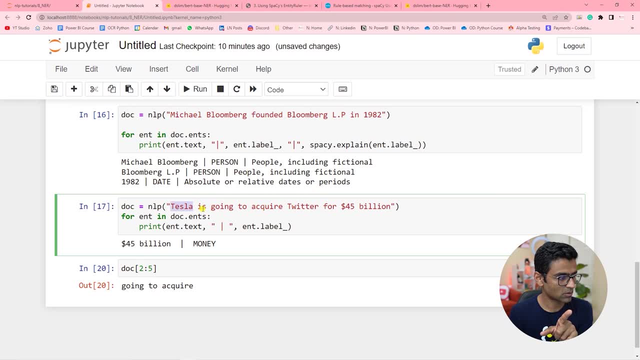 the way it works is: it starts with index two, so see 0, 1, 2, so see it going, going three, four, so it doesn't go all the way till five. it follows the usual Python convention. so start with zero, start with two, go all the way till five. button, do a. 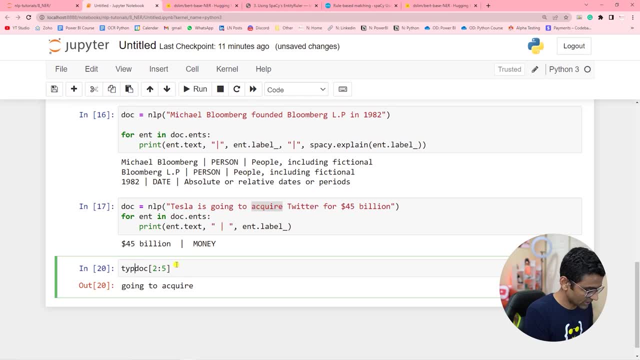 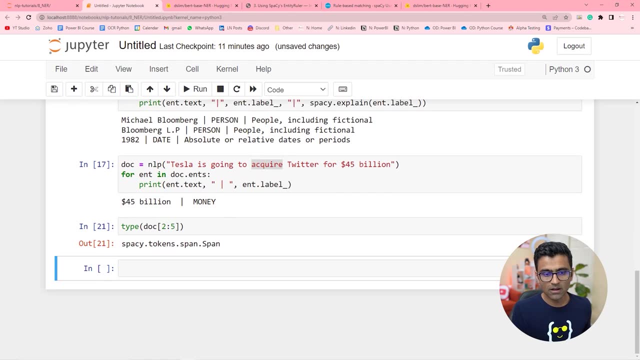 not include file and if you look at the type, see it is span, not spam. you can import this span class from spaCy and what you can say is my t1 or let's say s1, my first span from this document, starting from 0 to 1. so when I say 0 to 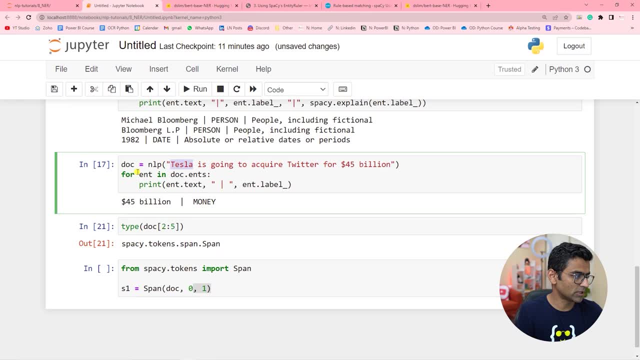 1, it is just one token, which is tesla. okay, so in this doc object 0 to 1, which is tesla. you're saying it is org and similarly okay, where is twitter? so twitter is 0, 1, 2, 3, 4. 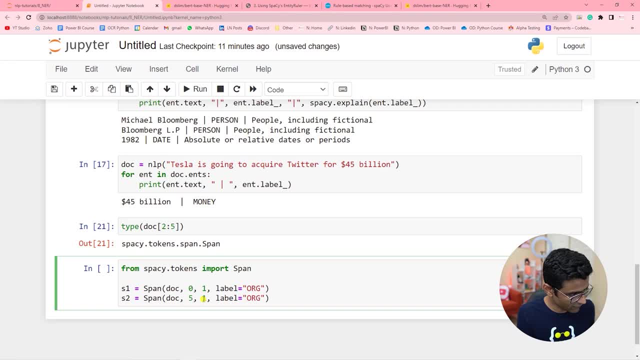 5. so 5 start from 5, go all the way 6, but do not include 6 and do. these two are my, my org entities and there is a function called setents. so on the doc you can set setents in the bracket. specify all the entities that you want. 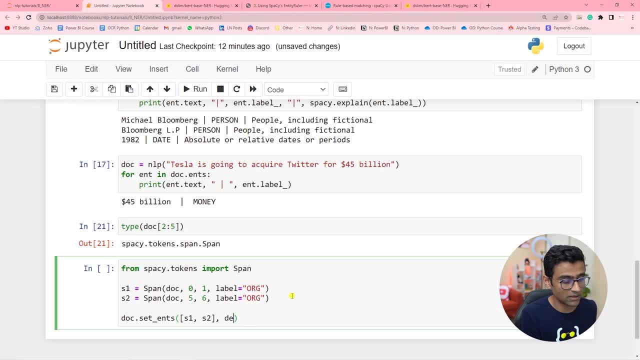 to set so s1, s2, and then say: default is equal to unmodified, so default is equal to unmodified. so default is equal to unmodified. so default on whatever default entities are there, you keep them as is and do not default on whatever default entities are there, you keep them as is and do not. 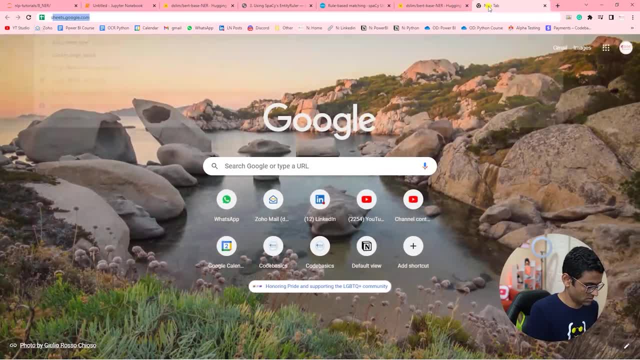 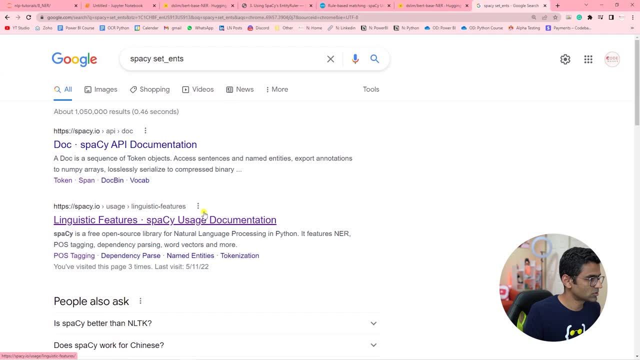 default on whatever default entities are there, you keep them as is and do not modify them. if you want to see a, modify them. if you want to see a, modify them. if you want to see a documentation, use your friend Google documentation. use your friend Google documentation. use your friend Google. spaCy said: ENTS shows you a. 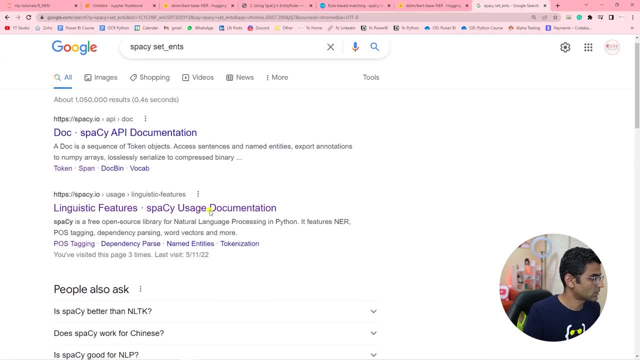 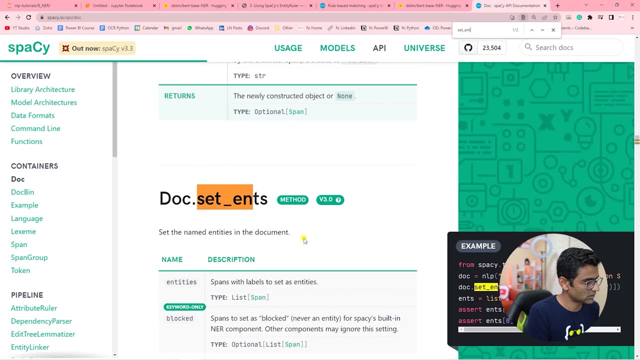 spaCy said ENTS shows you a spaCy said ENTS shows you a documentation somewhere I don't know documentation somewhere. I don't know documentation somewhere I don't know, where this Google is not recognizing it, where this Google is not recognizing it, where this Google is not recognizing it properly. so, on the doc, maybe said ENTS. 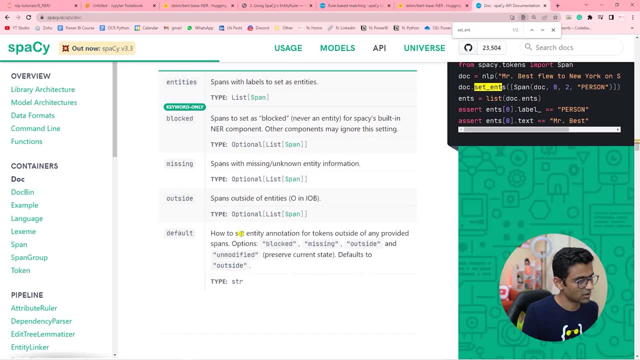 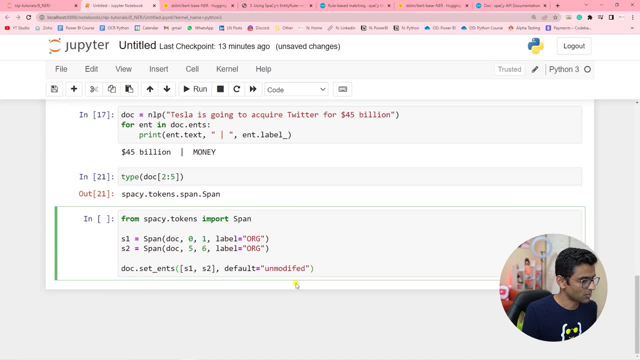 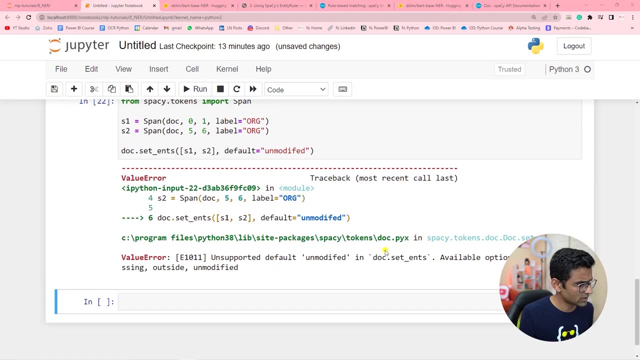 properly. so on the doc maybe said ENTS properly. so on the doc. maybe said ENTS this: okay, how to set entity annotation for tokens outside of any provider span. so you can read through the description. but this will basically set those two entities so unmodified. default is unmodified. there was a spelling mistake. 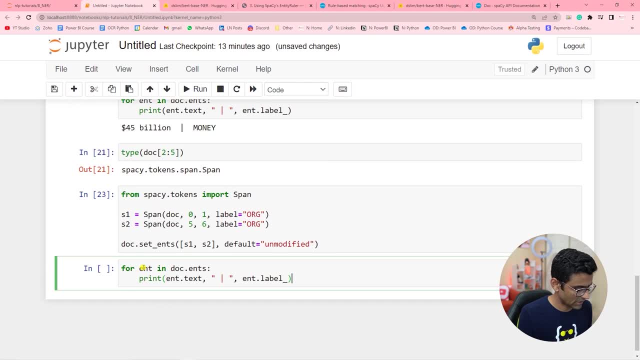 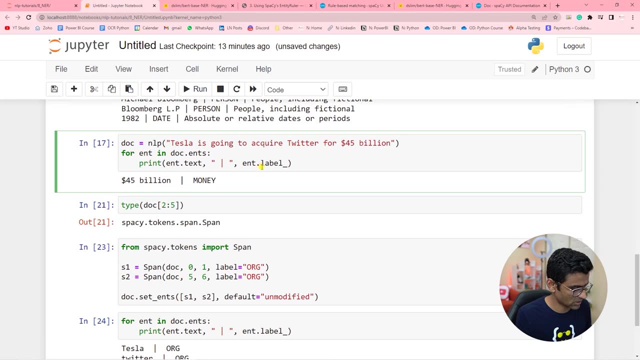 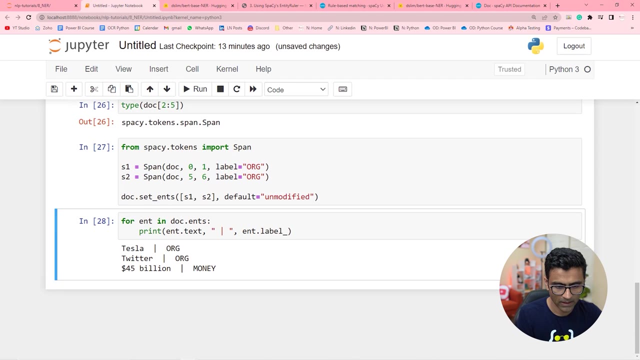 and when I print the same entities again now it is recognizing Tesla and Twitter as an organization. okay, so I can just read on it again, because there are T, that that you know. I fix the spelling for T now. I showed you how to use spaces- inbuilt capabilities of NER. but let's 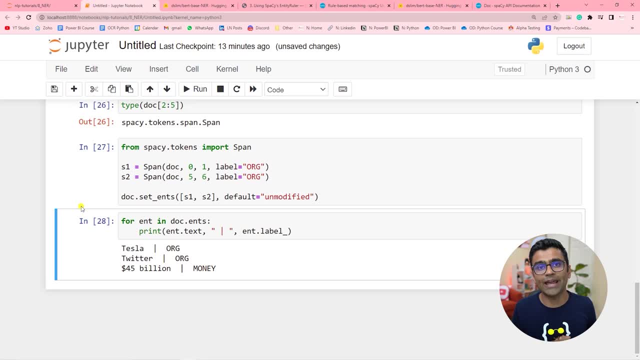 say you want to build your own NER system because we saw the out of the box NER system has some bugs, some issues. let's say you are having a pharmaceutical data set and you want to set entity for a drug. you need to do certain things so that you can train. 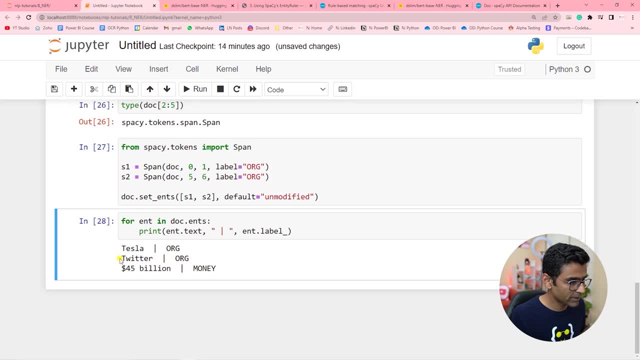 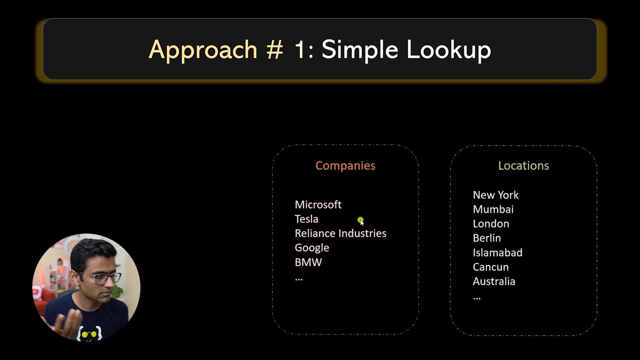 your own model. so I'm going to go very brief into that. so how can I build my own NER? the first approach is simple: lookup. so this is not a. some people say this is not an NER. this is not. this is a simple, hard-coded approach you can have. 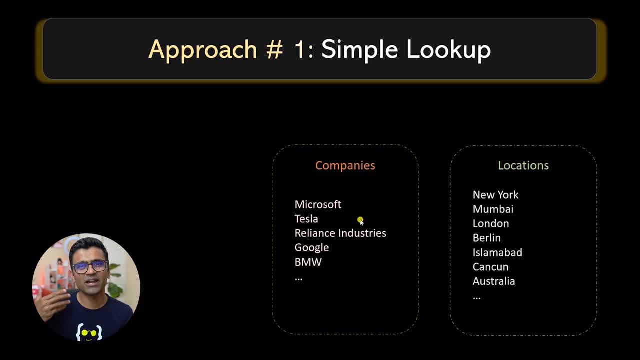 a database of companies, location, drugs, and as you get more companies or location or drugs in your vocabulary, you have a process where a, an operator, manually adds that entity into these databases and when you look at the tax and tokenize it, you do comparison. it's like a very stupid, very naive approach. 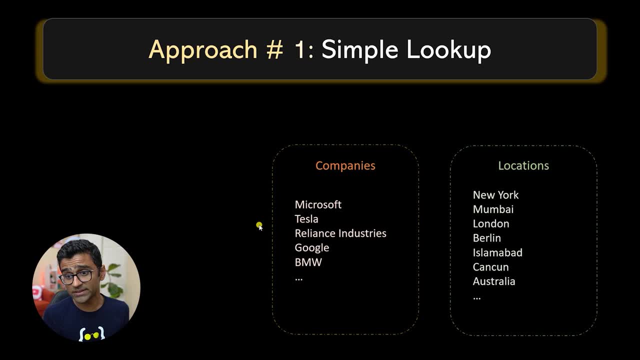 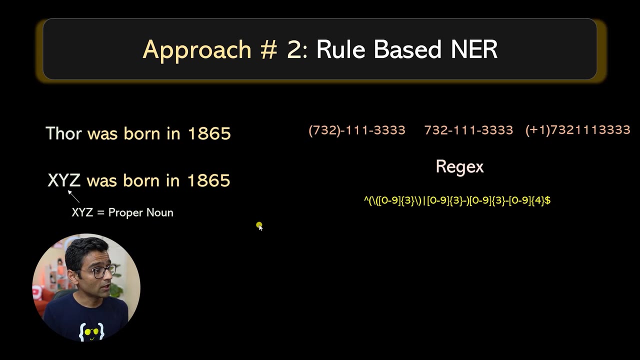 but it works. so some folks use this simple lookup and you know, as long as it works, you don't need to have unnecessary emotional attachment. for NLP or machine learning depends on your use case. maybe for your use case, simple lookup is the best idea. the second approach is rule-based NER and we saw already in. 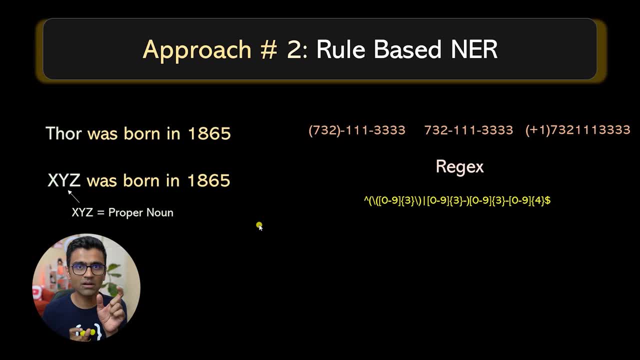 spaCy that it was using some rule that if there is a word followed by INC and the first letter of the word is capital, that is a company. similarly, let's say, if there is a statement like this: Thor was born in 1865. however, I don't know the real birth date of Thor- then you 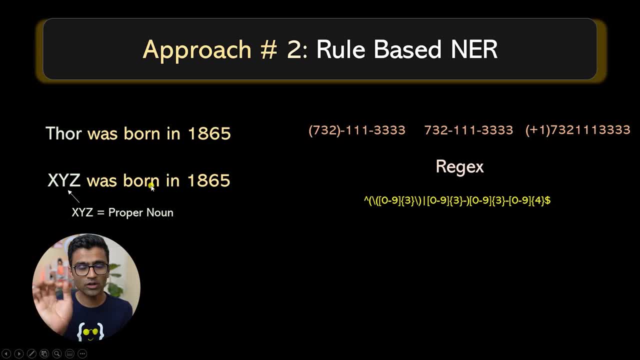 can say if you find this kind of pattern was born in something and before was, if there is a proper noun- we looked at POS before, so if you're not seen that video, go check it out. so if that is a proper noun, then that token is person. you can. 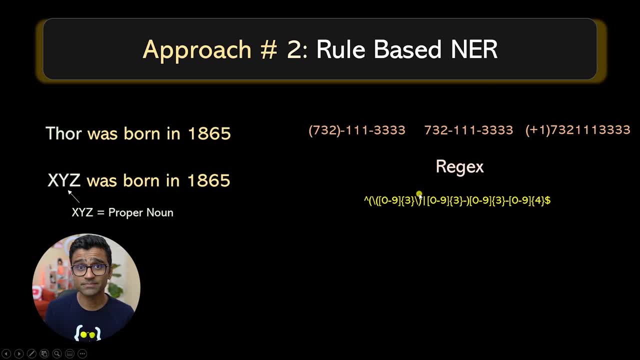 have that kind of rule. you can have a rule for phone numbers, for phone number based thing is regular expression. 就 Zoom, Doctor Ок. we already covered Regex in this tutorial playlist so anyone can see Regex or any other rules. but there are basically rule-based NER and spaCy provides a class called entity ruler that can be. 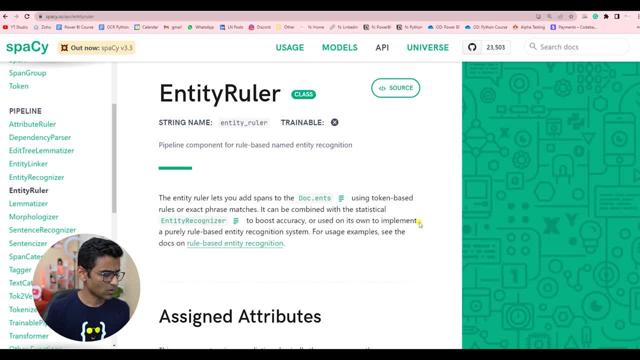 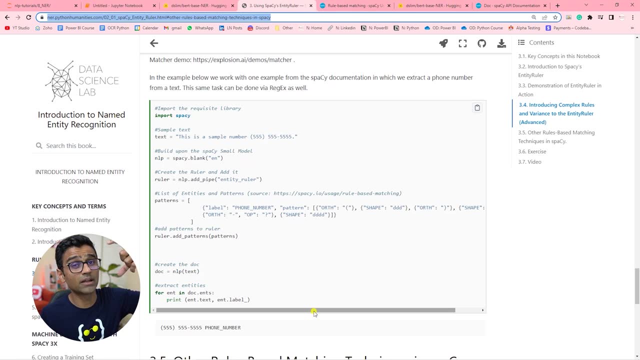 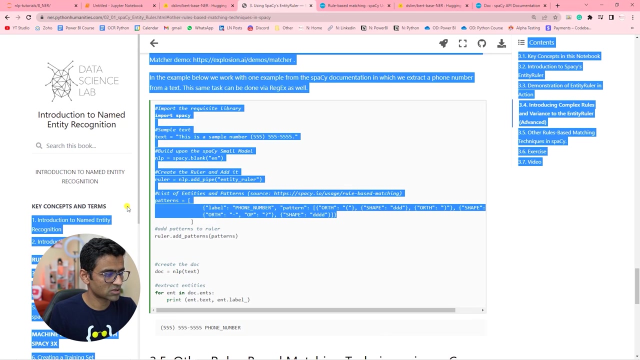 used to write or specify all these rules. ok, and I found this nice article which open süph Sen hopul to show you guys. so the article description is that article link is there in the description. so see here. to recognize phone number you can use entity rural class and you can specify your pattern like this: there's just a. 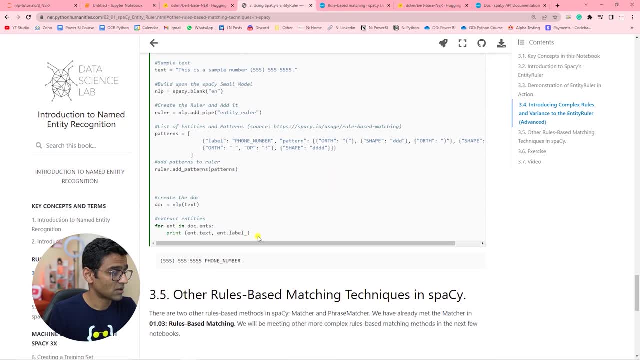 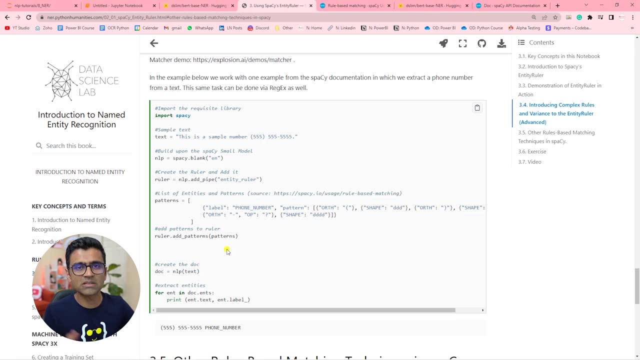 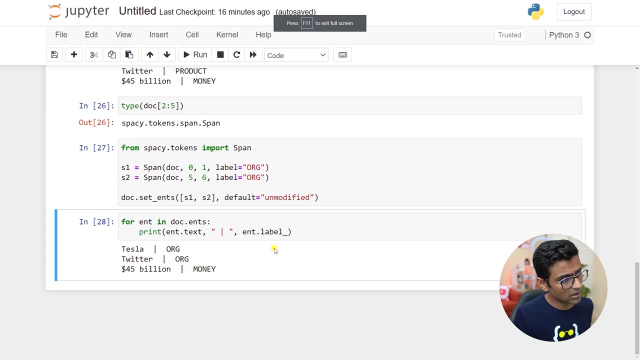 syntax that you can use to specify that pattern. and when you do that, see it says phone number. this is a phone number. I'm not covering this because this is just the basics of any are. in the future maybe we will build our own any, our system. I'm thinking of building a resume, a parser as a, as a project. so in the 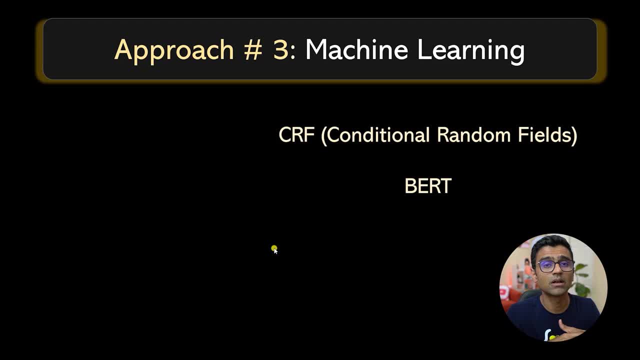 future we will have end-to-end NLP project in this playlist where we will use any are and specie to custom train our model. but yeah, the third approach is machine learning, where you can use a technique called conditional random fields. now, I know I don't like to use.